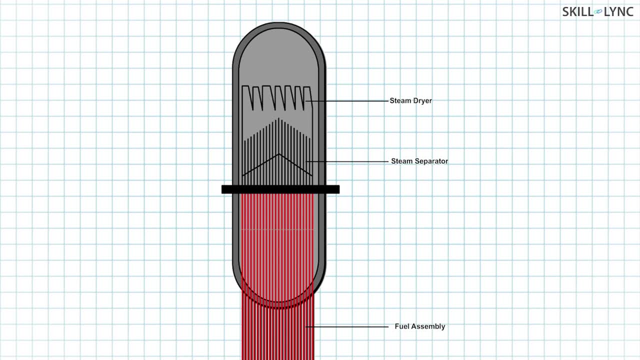 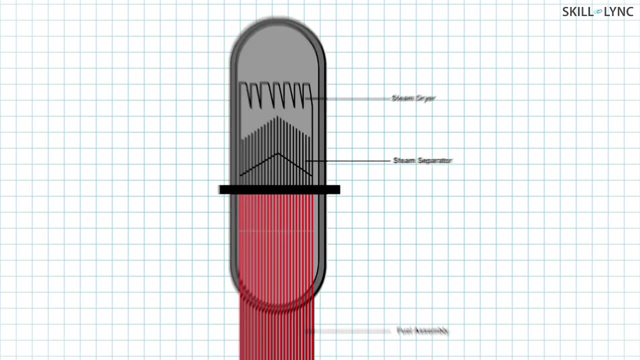 at the top of the vessel, the steam is separated from water and goes to the dryer, after which it drives the turbine. on the other hand, the water separated is sent back to the feed water. controlling the nuclear reaction in a boiling water reactor can be done in two ways: by using the control rods. 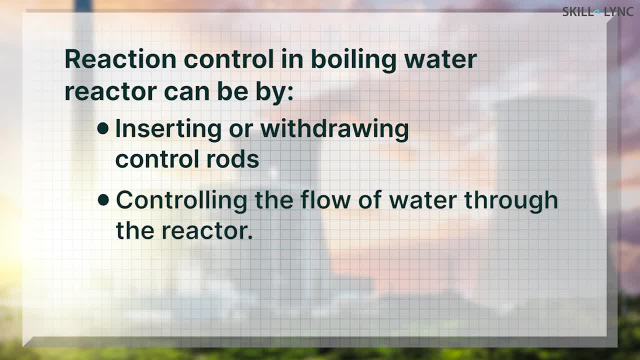 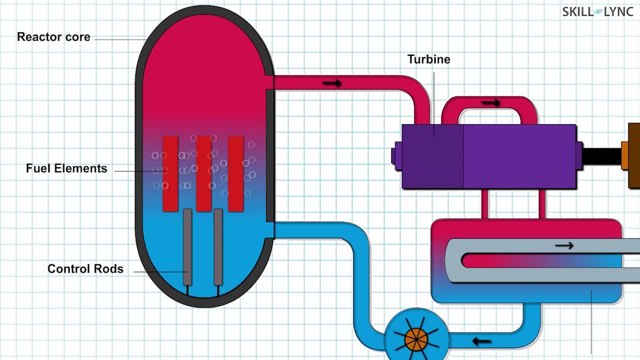 or by controlling the flow of water. when the control rods are used, they can increase or decrease the reaction rate based on their position. to increase the reaction rate, the control rods are withdrawn, while to decrease the rate, the control rods are inserted into the core. when the flow of 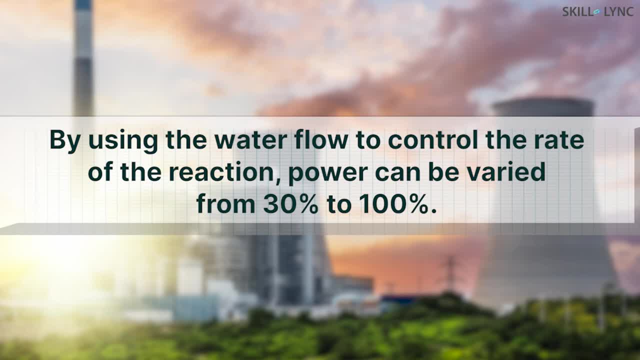 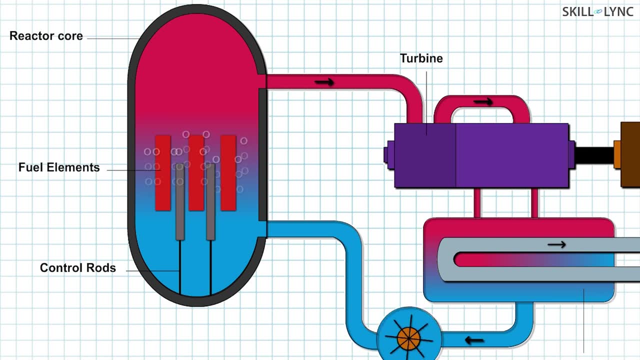 stormwater reaches the reactor, Darlington reaction rate can be used to vary the power from thirty percent to a hundred percent. when the water flow to the reactor core increases, the bubbles formed due to heat are taken away quickly. this makes more room for the water. now, since water is a 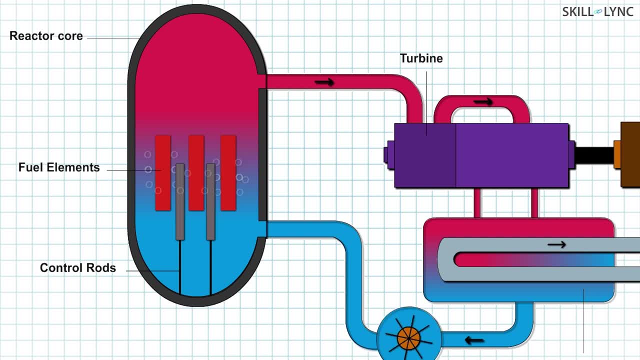 neutron moderator. it slows down more neutrons. that has to be absorbed by the fuel. this increases the rate of the reaction. but when the water flow to the reactor cord decreases, the bubbles stay for a long Well, that's all about the working of a boiling water reactor. 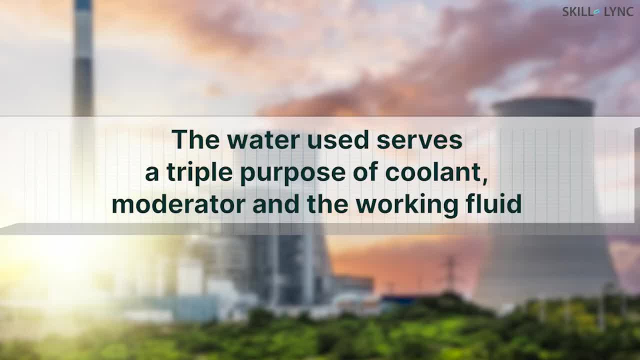 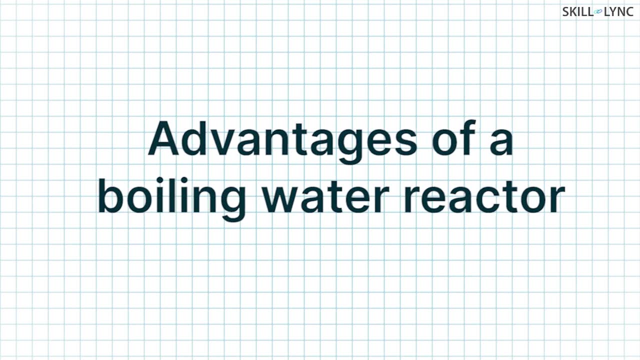 One interesting thing about the boiling water reactor is that the water used serves a triple purpose of being a coolant, a moderator and a working fluid. Now let's discuss some advantages of a boiling water reactor. The operation of a boiling water reactor takes place at a lower pressure. 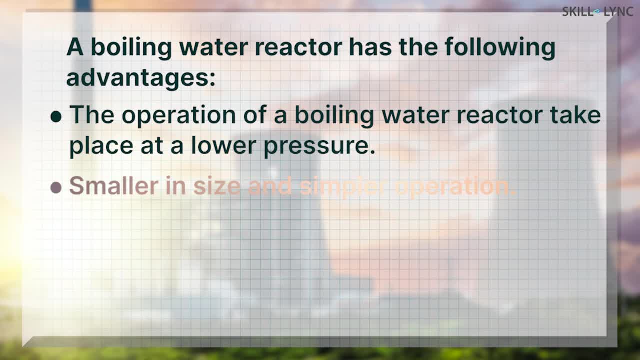 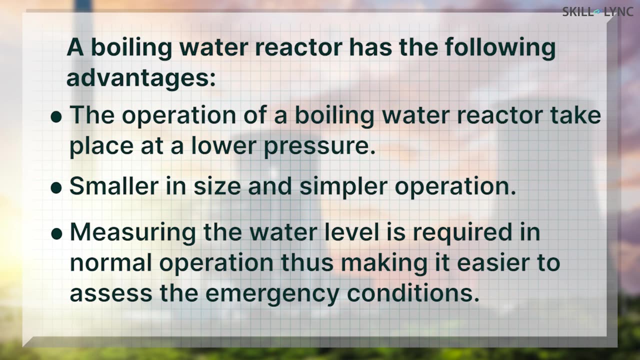 as compared to a pressurized water reactor. Secondly, there is no use of a pressurizer or steam generator, Therefore, the operation becomes simpler and the size smaller. The water level should be measured to assess the emergency condition, Since a boiling water reactor requires measuring of water level even in normal operation. 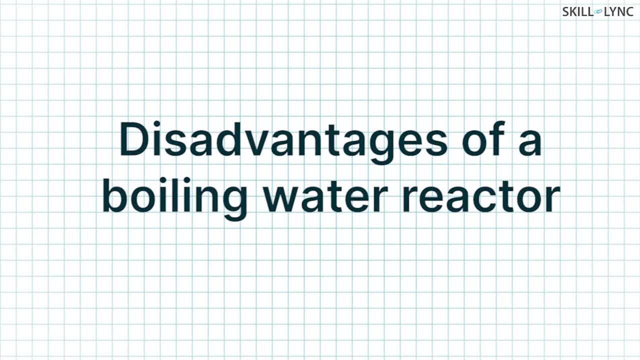 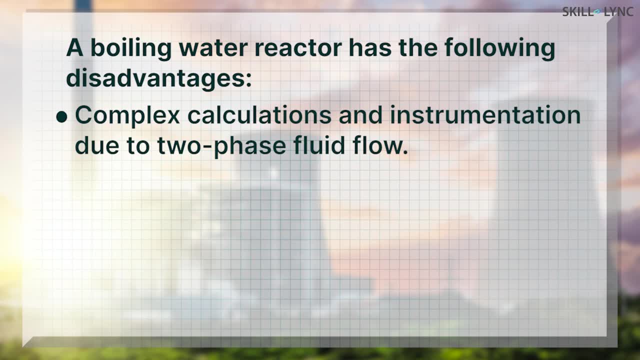 the possibility of accidents are reduced. While there are advantages to boiling water reactors, there are also some disadvantages. First of all, the boiling water reactor works in a two-phase fluid flow. That means both water and steam are present. This makes the instrumentation and calculations a bit more complex. 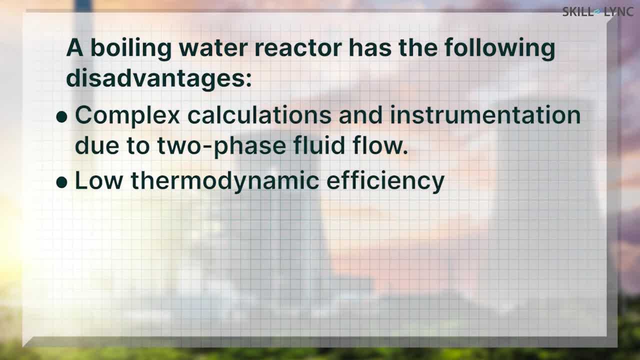 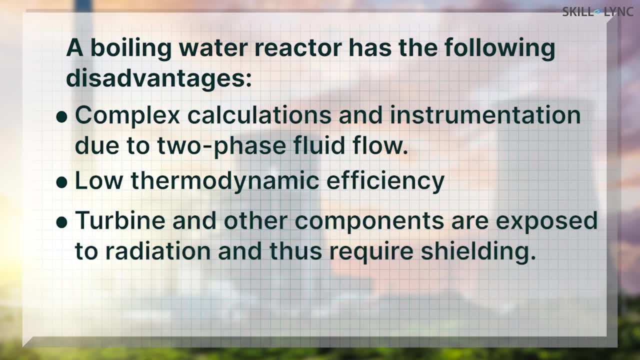 Secondly, the boiling water reactor operates at lower pressure than a pressurized water reactor, Thus giving a low thermodynamic efficiency. Thirdly, since the steam to the turbine enters directly from the reactor core, it is exposed to radiation as well.